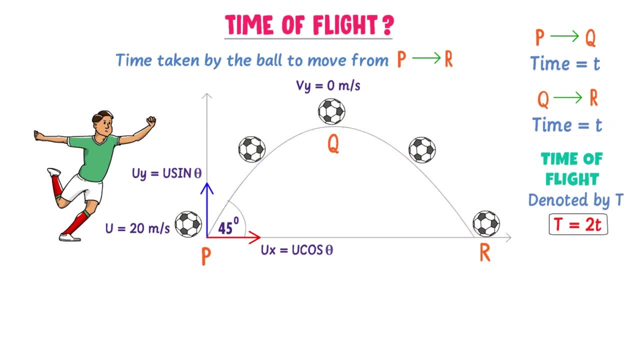 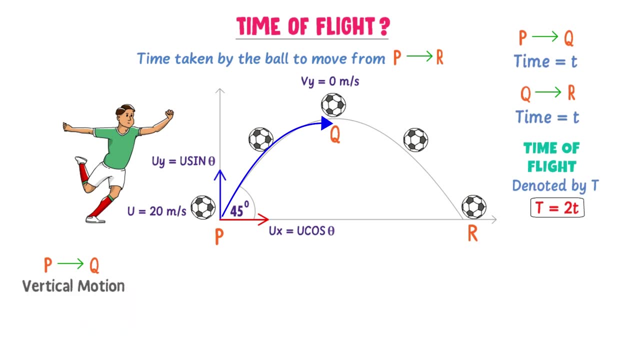 t, it goes down. Now I am interested to find the time taken by the ball to reach maximum height from p to q. Hence I consider only the vertical motion of the ball. We know that the initial velocity of the ball in y direction is ui. 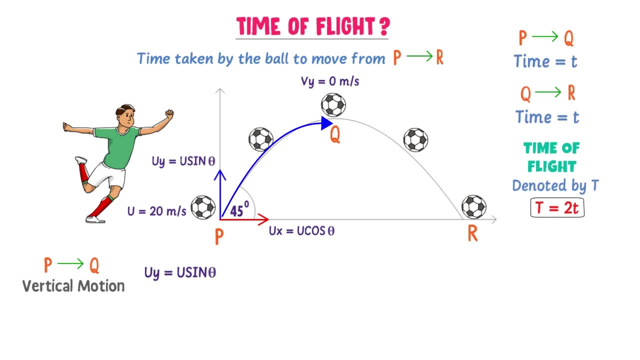 is equal to u sin t And the final velocity of the ball at q. our maximum height is. vy is equal to 0 m per second. Also, the acceleration a is equal to negative g and, as mentioned, I am interested to find the time taken by the ball to go from p to q. 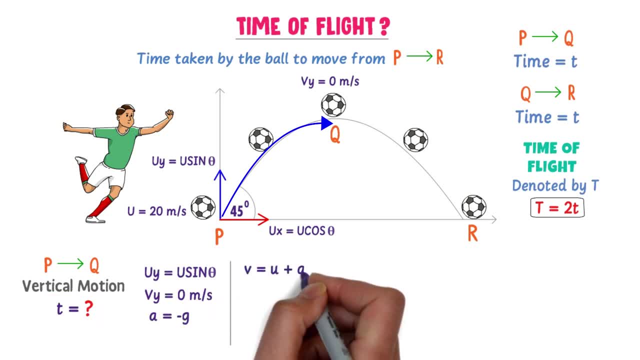 We know that these all parameters are joined by the equation: v is equal to u plus at The final, velocity v of the ball is zero, The initial velocity u of the ball is equal to u sin t And the acceleration of the ball is negative g to t. 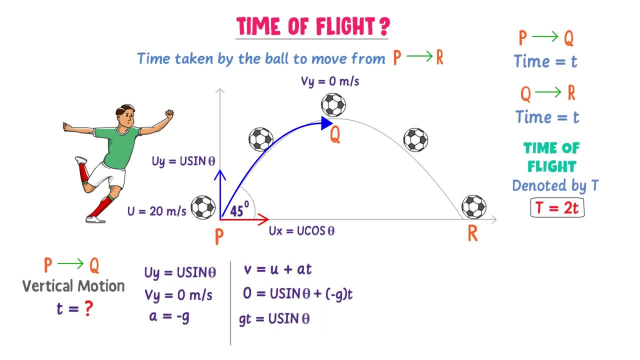 Rearranging the equation. gt is equal to u sin t, Rt is equal to u sin t upon g. So the ball will take. t is equal to u sin t upon g. time to go from point p to point q. Now it will again take. t is equal to u. 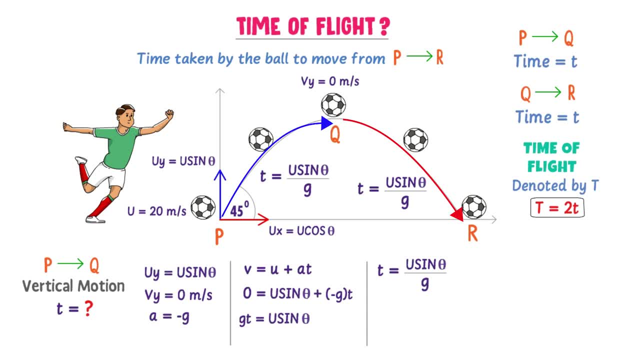 sin t upon g time to go from q to r. Now how much time it will take to move from p to r, p to r. well, we know that t is equal to 2 times smaller t, So the time of flight of the ball is. 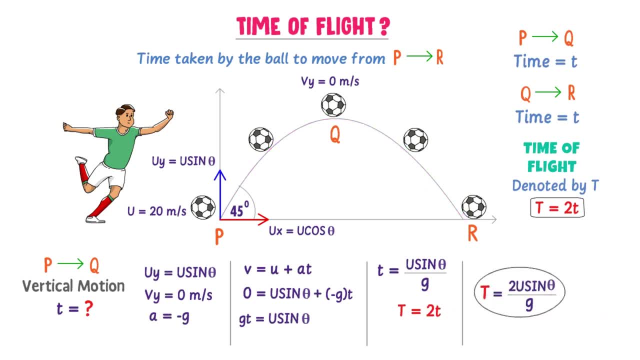 t is equal to 2 u sine theta upon g. This is the equation of the time of flight of a projectile. Also, let me teach you one another method of deriving the equation of time of flight of a projectile. Consider the vertical motion of the ball from p to r, The initial velocity of the 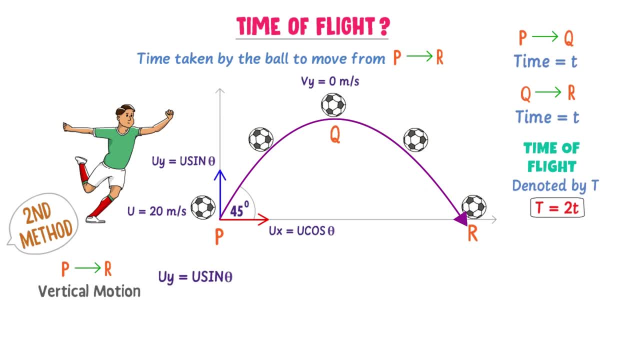 ball in vertical direction is: ui is equal to u sine theta. Acceleration a of the ball is negative g. The displacement of the ball in vertical direction is sy is equal to 0 meter. Let me explain this. Consider that a ball is present on x-axis and its x-coordinate is 1 and y-coordinate. 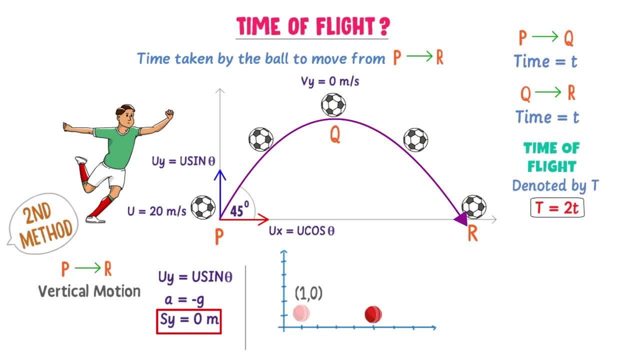 is 0.. Now the ball moves to this point. Here its x-coordinate changes to 5, but its y-coordinate is again 0.. Thus we say that this ball is displaced along x-axis direction because its x-coordinate changes from 1 to 5.. But the ball has zero displacement in y-direction because its y-coordinate doesn't. 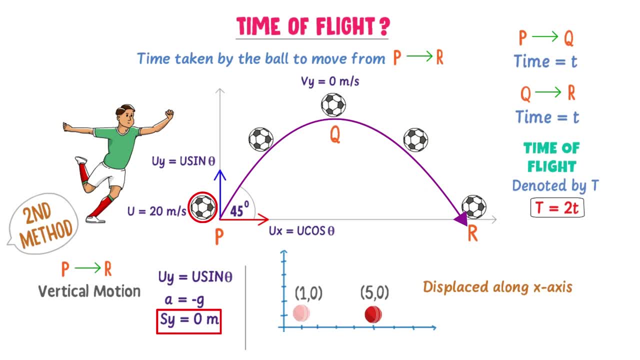 change. Similarly, at point p, the ball is present on x-axis. At point r, the ball is again present at x-axis. So this ball is displaced in horizontal direction from p to r, but vertically its displacement is 0. Now I am interested to find the time of flight of the ball to move from p to r. Hence these: 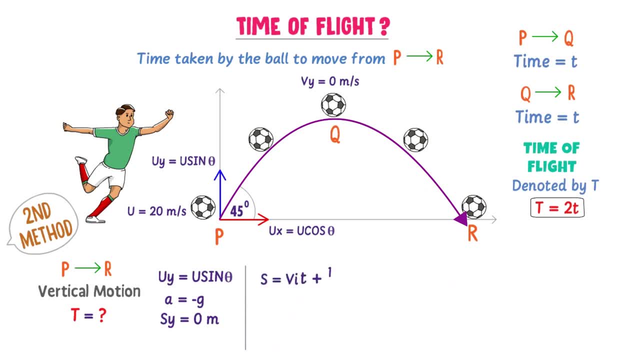 all parameters are joined by the equation: s is equal to vit plus half at squared. We know that the displacement sy is equal to 0.. Initial velocity of the ball is u sine theta into t plus half negative g into t squared. Now we take t common, as 0 is equal to t into. 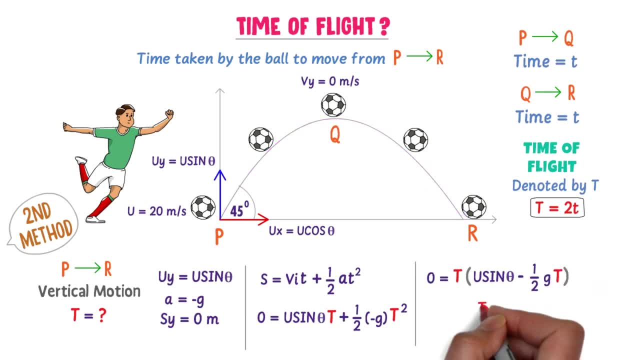 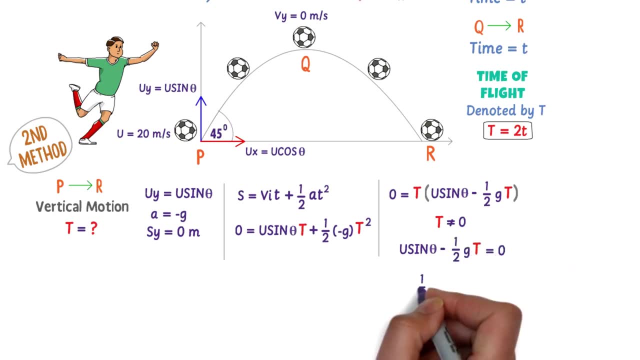 u sine theta. We know that t is not equal to 0.. So, u sine theta, minus half gt is equal to 0, or half gt is equal to u sine theta, or t is equal to 2, u sine theta upon g. Hence this is the equation. 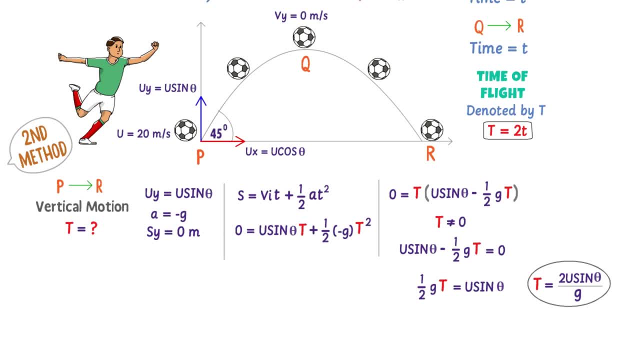 of time of flight of the ball. Now let me use this equation to calculate the time of flight of the ball. The initial velocity of the ball is: u is equal to 20 meter per second, The angle of projection is 45 degree and acceleration due to gravity is 9.8 meter per second squared. We know that. 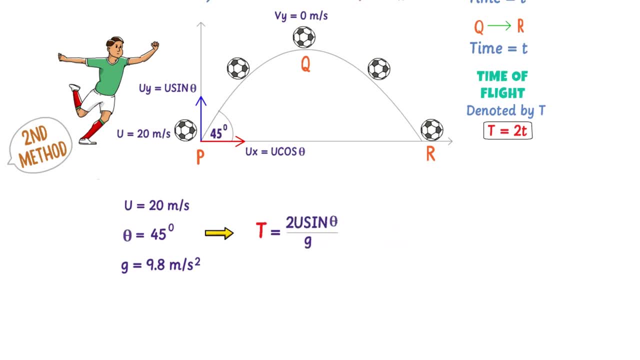 the time of flight. t is equal to 2 u sine theta upon g. Plug in all these values in this equation we get t is equal to 2.9 second. So the ball takes 2.9 second to move from p to r if you throw it with initial velocity of 20 meter per second at an angle of projection. 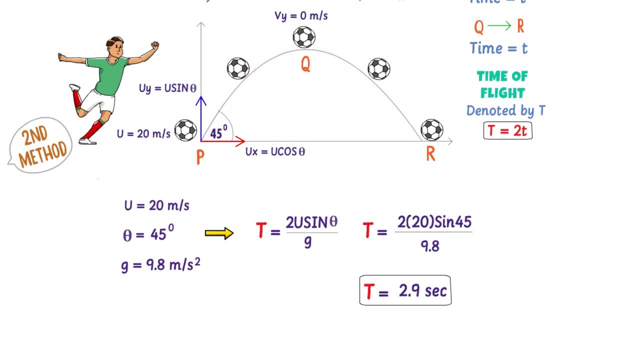 of 45 degree. I hope that you have understood this video. If you have any questions, please comment below. Thank you very much for watching this video.